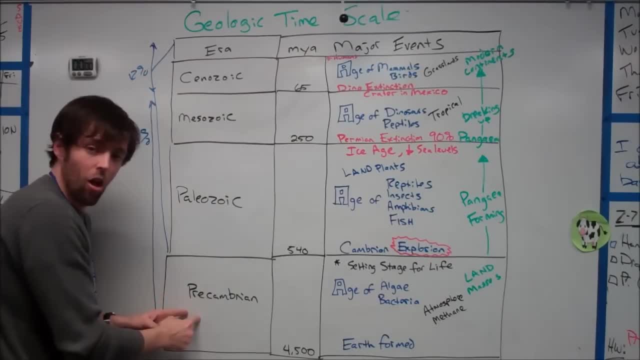 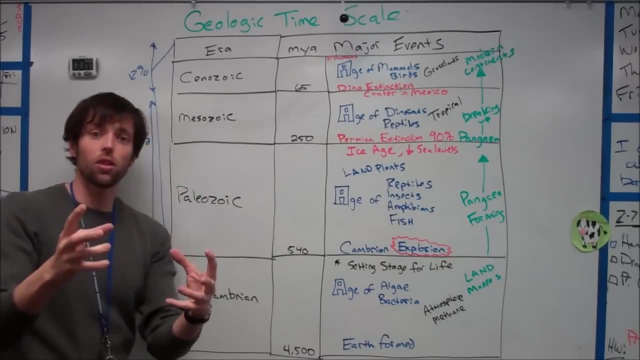 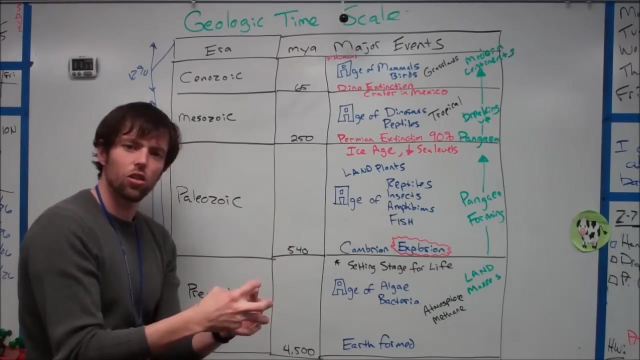 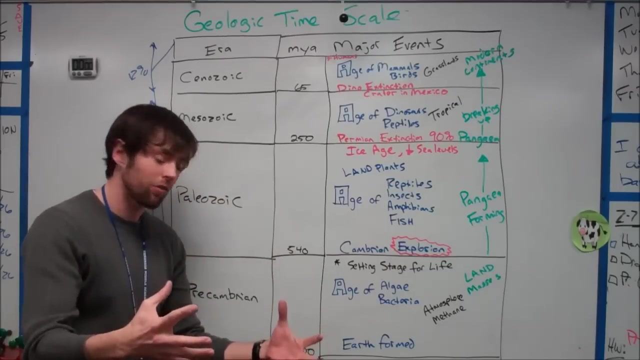 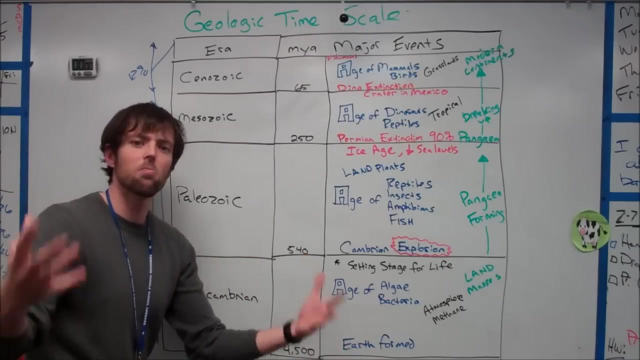 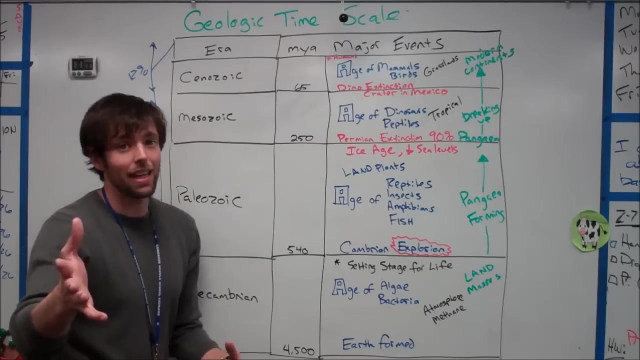 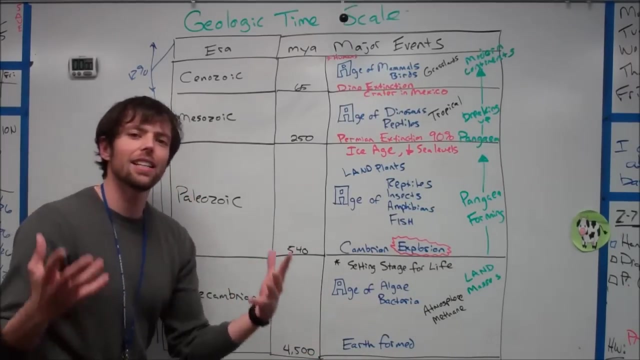 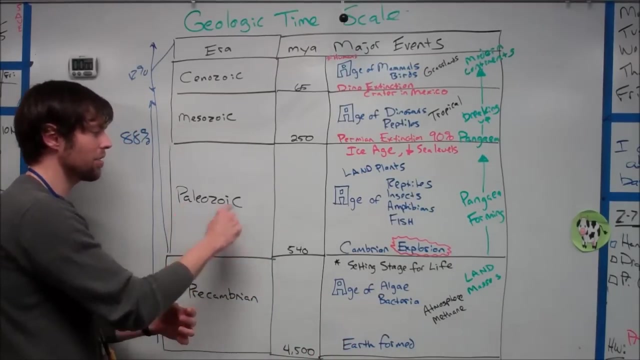 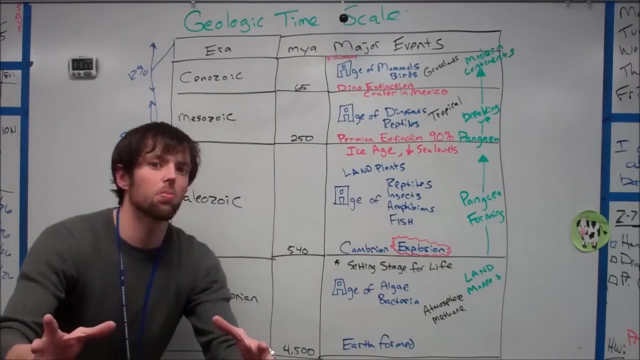 That's crazy. So what happened during the pre-Cambrian? Well, all this dust and debris was flying around in outer space and sort of... glommed together due to gravity and intermolecular forces out in space. And as it spun around the sun, the moon was kicked off, and all these heavy metals were sinking into the Earth's core, and eventually we have land masses, and we have volcanic activity, we have meteors hitting from outer space, until eventually some reason bacteria was like, this sounds awesome, I'm gonna come to life in these primordial old oceans. And the atmosphere was stinky, it was full of helium, but especially methane, a gas we don't have today, and as time went on, just billions of years, even with this bacteria, it was setting the stage for life. And life came about as we transitioned to our next stage, the Paleozoic, or early life. An event occurred called the Cambrian explosion, and it wasn't a bad explosion, it was a good explosion, it was an explosion of all of these guys into the world. 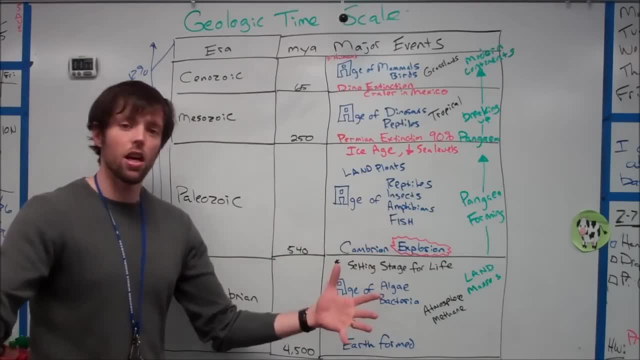 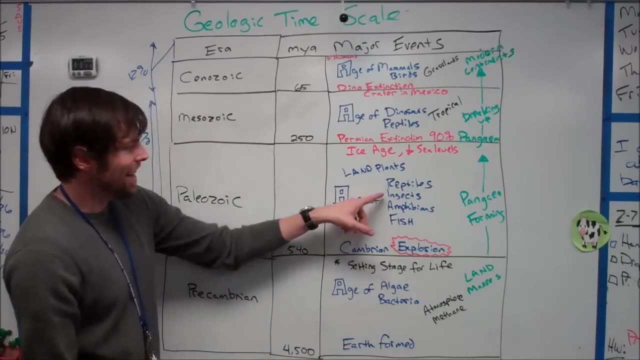 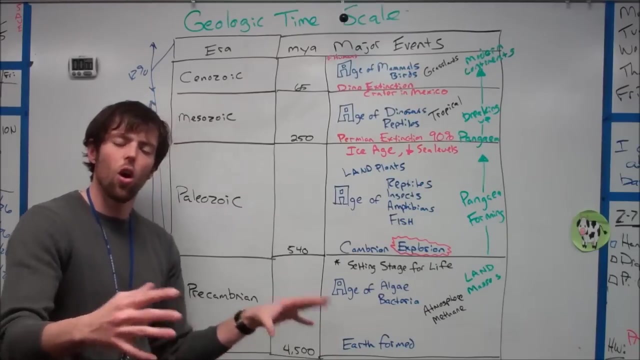 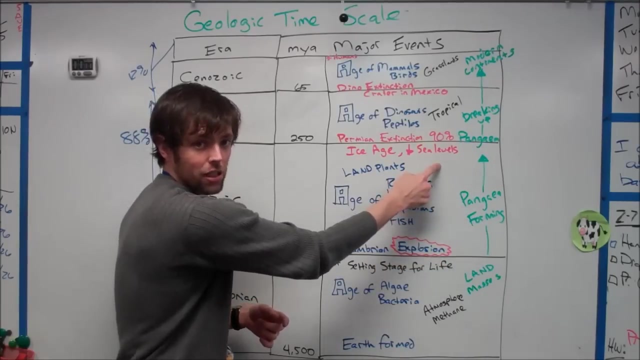 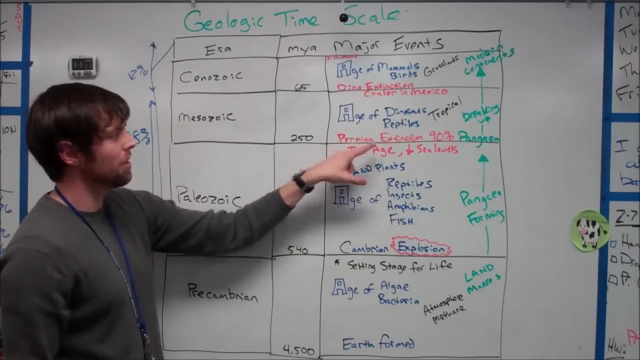 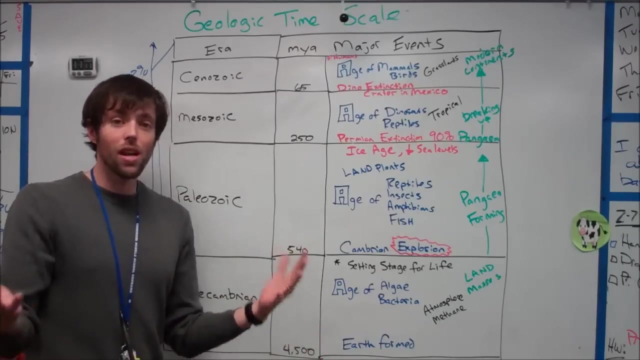 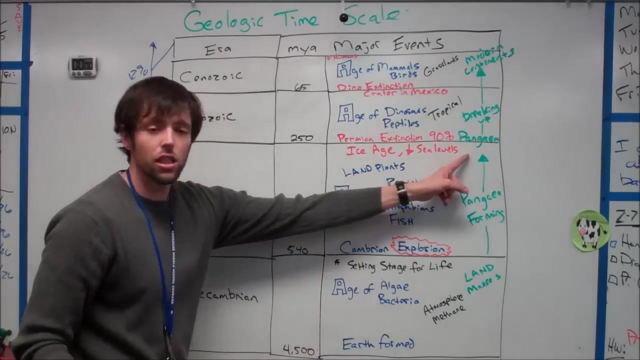 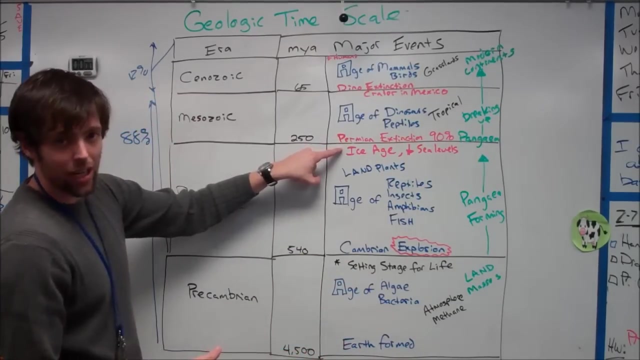 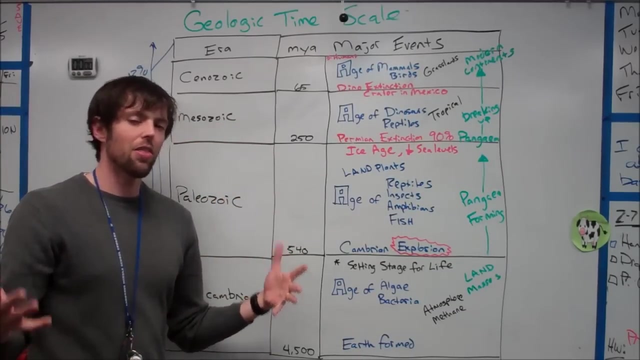 And all of a sudden, bacteria... longer the only ones in the ocean. There was fish in the ocean, and there were amphibians in the ocean, and then on land there was finally land plants occurring, and insects, and by the end there was even reptiles. And as this was occurring, all these land masses that were being formed from the crust were starting to come together to form this huge supercontinent that you and I know as Pangea. So that was forming during the Paleozoic. By the end though, something crazy happened. This extinction event we call the Permian extinction occurred, and 90 percent, 90 percent of all living things was just wiped out. We're not totally sure how this happened. We think it might have been due to an ice age occurring at the time that caused sea levels to drop. Maybe it was Pangea forming. We're not exactly sure. There was oxygen levels in the atmosphere that were fluctuating, but this ushered in a new age we call the Mesozoic age, or middle age. And during that age, there were reptiles that really came to flourish. And this is that classic age of dinosaurs that you think about. It was tropical by the middle of the era, and Pangea started to break up into these larger supercontinents. But then by the end, a huge meteorite came and blasted into Mexico, threw all this debris into the air, and what we know is that the dinos didn't make it. 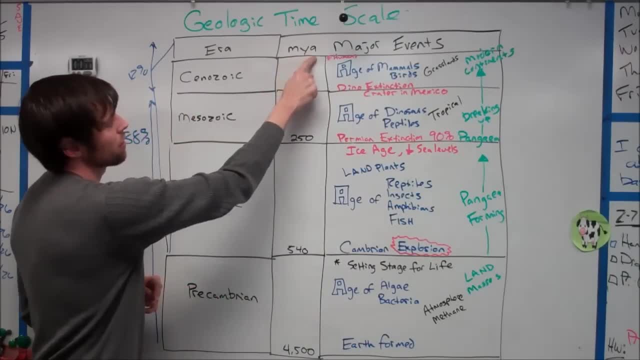 And so a bunch of them died off 65 million years ago, which ushered us into our final age, the Cenozoic.